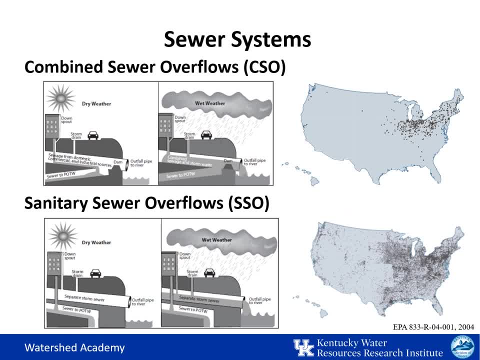 water bodies untreated. The graphics indicate where these different types of overflows occur with the United States. Combined sewer overflows, or CSOs, are designed so that storm water flows into the same set of pipes as sanitary discharges. During heavy rains, excess flows go into streams at designated locations. 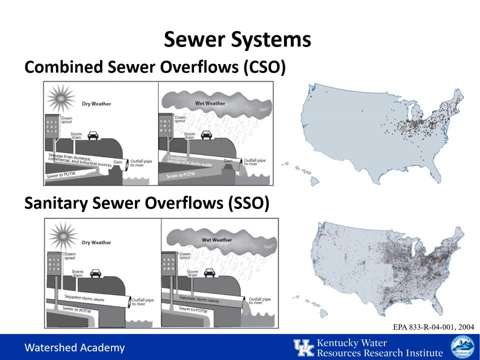 In separate systems. the rainwater is supposed to flow into storm pipes that are separate from the sewage. Unfortunately, water infiltration into leaky or cracked sanitary sewer pipes can cause sewage overflows as well as blockages. The maps show where these overflows occur. 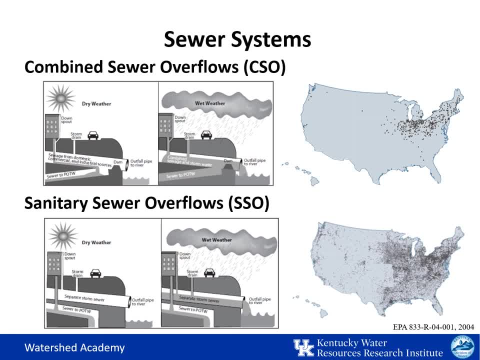 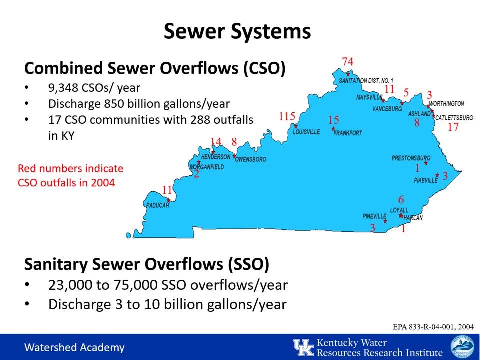 SSOs are much more numerous than CSOs. however, CSOs contribute much larger volumes of flow and associated pollutants. The maps and statistics on this slide and the previous slide are from the 2004 NPDES CSO report. A number of these CSOs have been corrected since that time, but this provides a state-level. 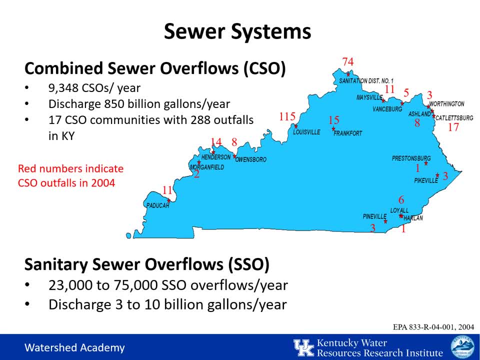 comparison between CSO and SSO volumes. As you can see, combined sewer overflows had 9,000, over четы of KG of CO2 discharges per year from 17 different communities and 288 outfalls. SAMHSA ver analyzes each of these positive systems for the circumstances of SDC offerings. 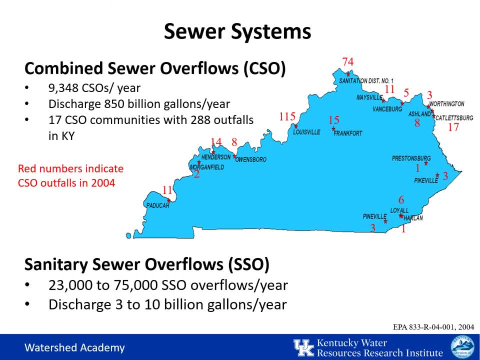 Forher CNV has provided the results of very comprehensive households for plagiarization and soil ERG applications such as S sowingsahoes, Thank you. sewer overflows: the number is much higher at 23,000 to 75,000 SSOs, that is, overflows per year. 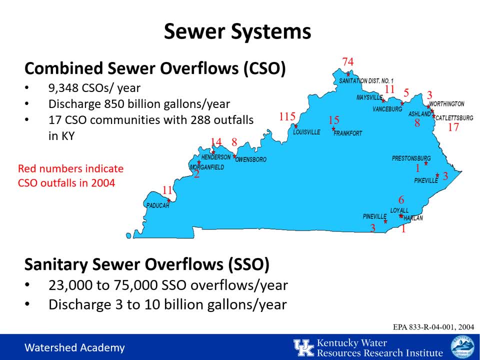 discharging 3 to 10 billion gallons per year. So many more overflows, but much lesser volume for the SSOs. So again, while SSOs are more common throughout the state, CSOs contribute much greater volumes of discharge. It's important to understand the type of sanitary system that is. 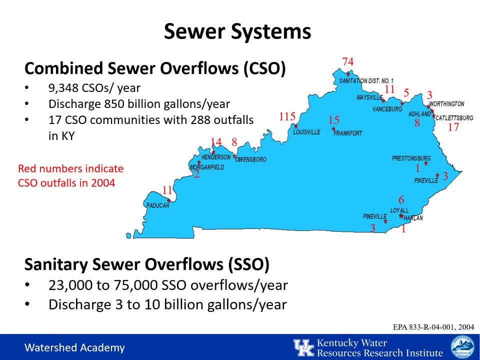 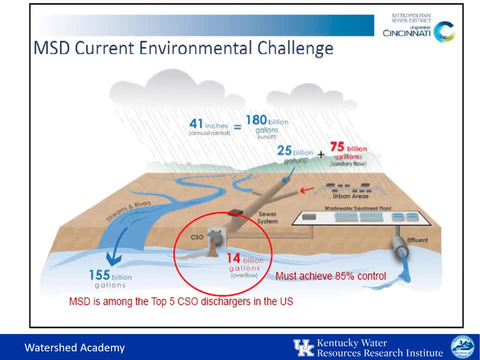 located in the watershed area in which you're working. This information will be helpful with developing appropriate management recommendations for water quality improvements. Here you can see some of the challenges in CSOs communities. This one is in the Metropolitan Sewer District of Cincinnati, one of the top five CSO dischargers in the United States. 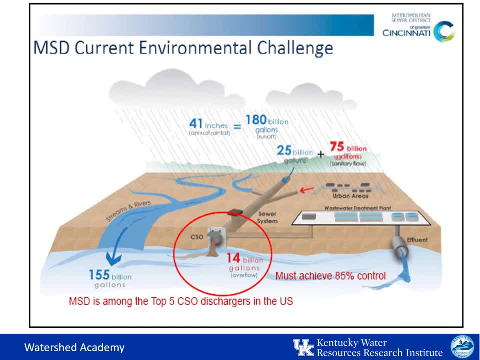 41 inches of rainfall produced 180 billion gallons of runoff. Of this, 155 gallons, or 86 percent, flows into the streams and the rivers, but 25 billion gallons enter the combined system. This accounts for 25 percent of the total volume that these sewers can carry: 14 billion gallons of this sewage or stormwater. 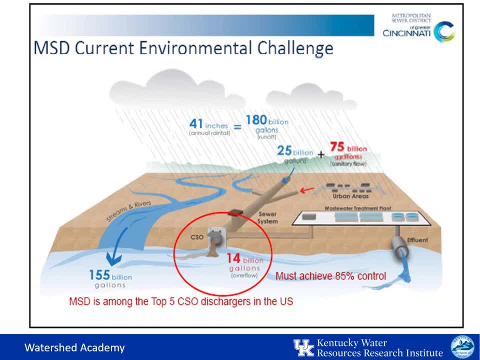 mixture overflow into streams, while 86 billion gallons are treated at the wastewater treatment point. The challenge is how to reduce the volume of stormwater entering the treatment process. The use of green infrastructure is one approach to reducing the amount of stormwater entering the. 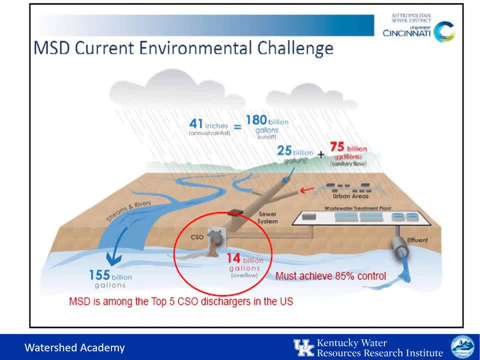 system. in these combined sewer system areas. Measures such as grass, swales or channels, rain gardens and vegetated parking lot islands help excess water to slow down and sink into the ground. It is also helpful to begin to separate the sand and the water from each other so that the 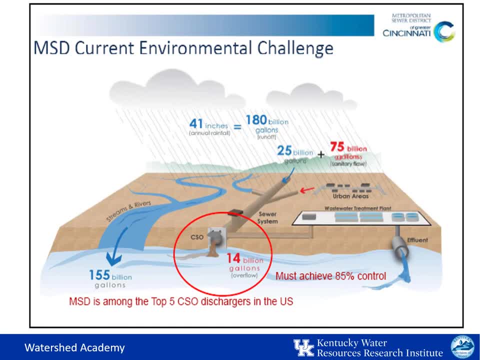 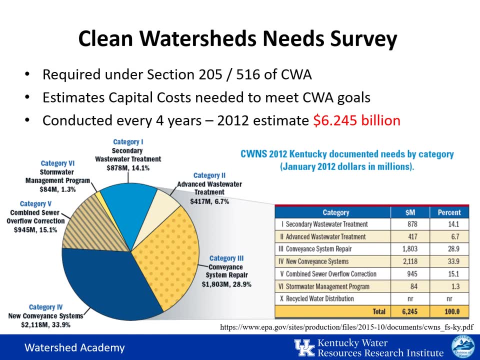 containers are not little scattered, Limit the dependence on previous system. Thailand: The DXA크 charge involves reaching out to data centers to raise Fördüttel Xe fermentable right water budget, which features resources from basic purposes rounds Eleunctioned data were not wishing, where possible. 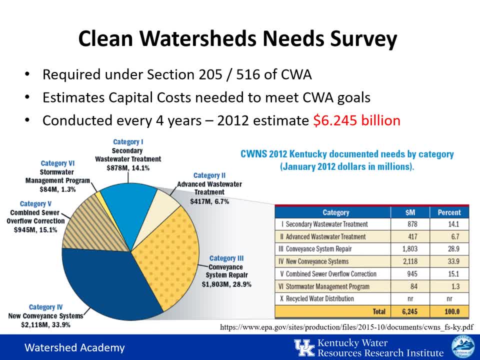 The Clean Water Act requires até ngày 2020, từ 2019 до 2020.. The Clean Water Act requires that each state estimate the capital cost required. dispose комментариях to meet the Clean Water Act goals for wastewater planning. 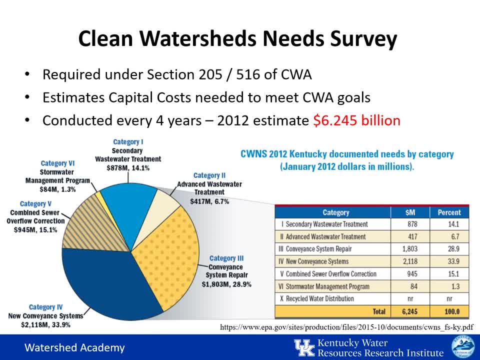 For concrete applications, the Clear Water Act requirement is 6. initial сум寸 Hy έχ � ar Salz e rebajen proposed costs previous meetings. The 2016 survey program was not available at the time at which this presentation 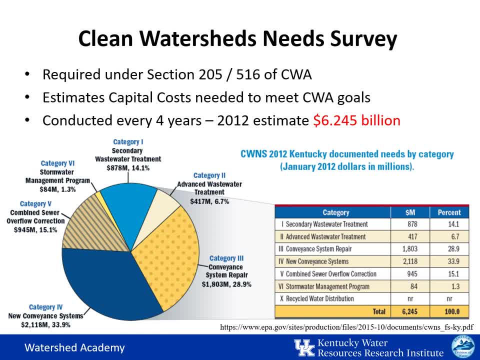 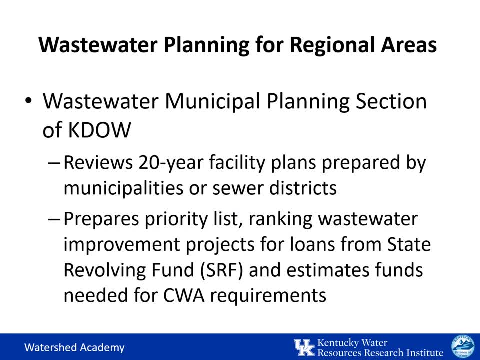 most expenses needed to address the wastewater system, repair, new systems and the correction of the combined sewer overflows. When working with wastewater utilities in the area, it is important to know what projects are currently proposed in your area and their ranking for potential funding. 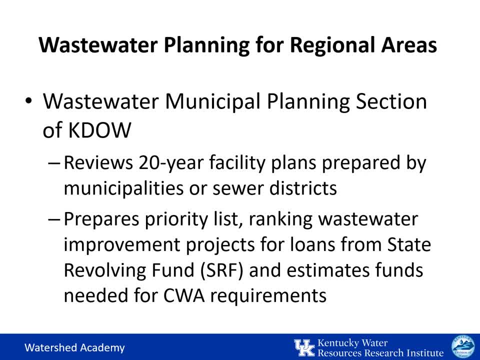 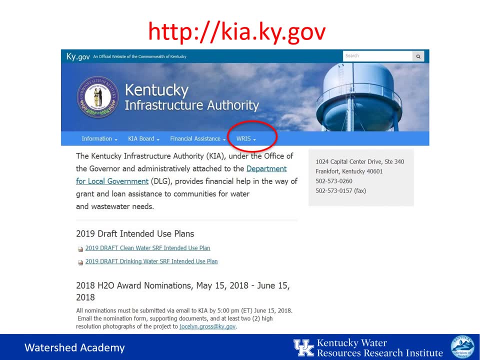 The Wastewater Municipal Planning Section at the Kentucky Division of Water reviews these plans with a 20-year projection in order to inform the Clean Watershed Needs Survey. If you would like to review this information, you can access it through the Kentucky Infrastructure Authority website. 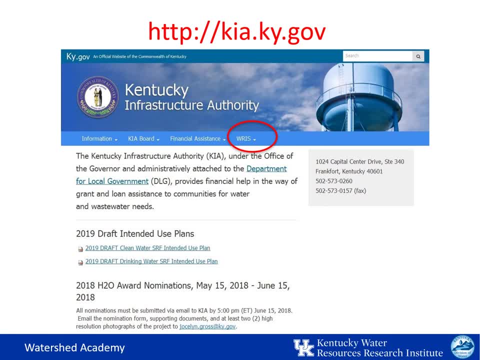 Under the WRIS tab, click the Management Plans option on the drop-down list and look for the Kentucky Wastewater Management Plan section. You can also review a lot of information about the Municipal Planning Section at the Kentucky Division of Water reviews this information. 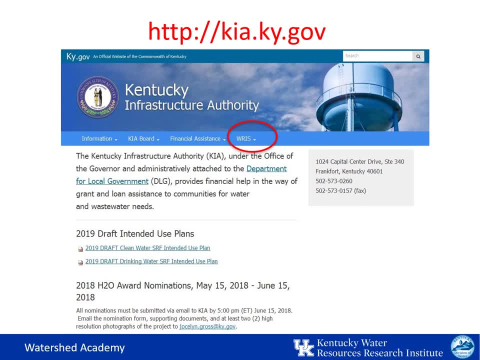 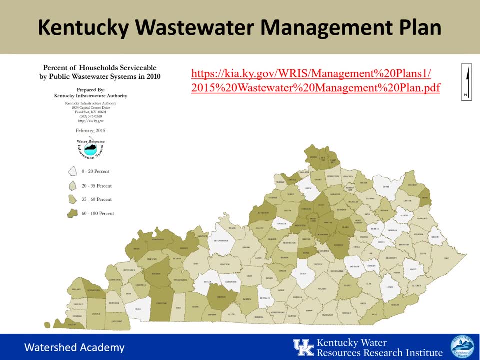 If you would like to review the Kentucky Wastewater Management Plan section, click the Management Plans option on the drop-down list and look for the Kentucky Wastewater Management Plan. In the Wastewater Management Plan you will find the percentage of homes that are serviceable. 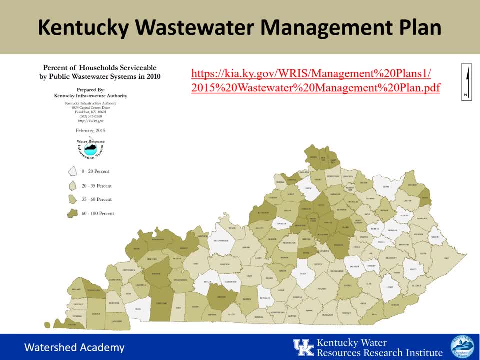 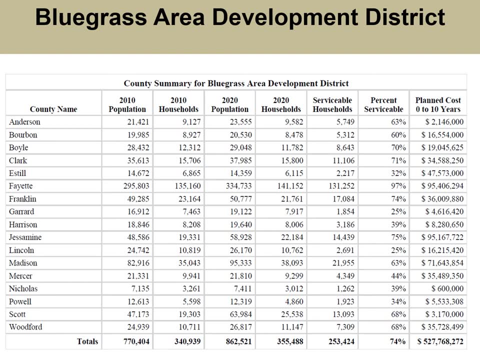 for public wastewater systems. This will give you an idea of the number of septic systems or straight pipes that you might find in your area. Here is another county level analysis within the Blue Grass Area Development District from that same wastewater management plan document. Particularly interesting is the percentage. 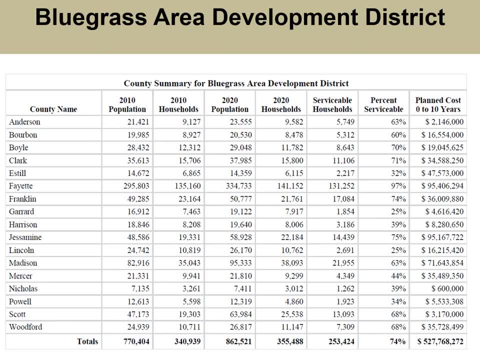 of serviceable households, meaning that these households could connect to municipal sanitary sewer lines. This will begin to help you to understand at a county level what the prevalence of sanitary sewer connections might be in the county as opposed to other connections. This plan also lists the proposed wastewater projects. 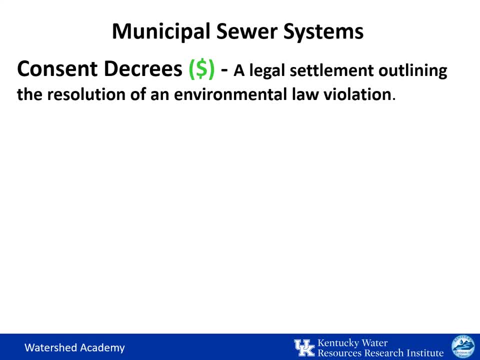 throughout the state To stop violations of the Clean Water Act. the EPA has negotiated a number of consent decrees for municipalities in Kentucky. These actions include large fines, required actions for the municipality and even outline projects that must be completed. As an example, Louisville, Kentucky, had a consent decree. 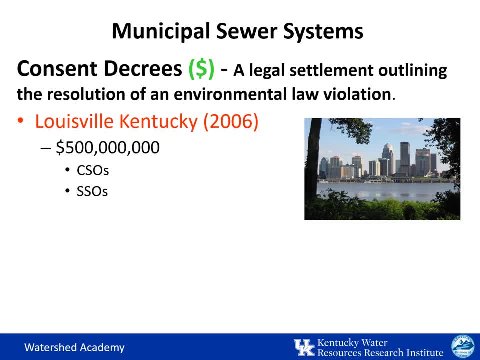 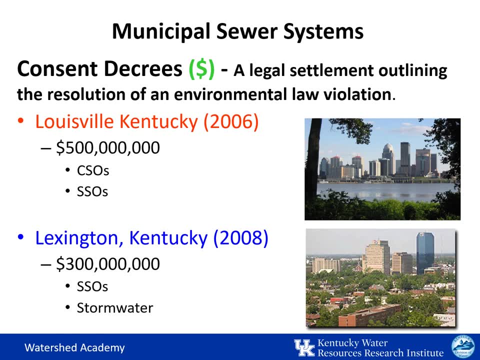 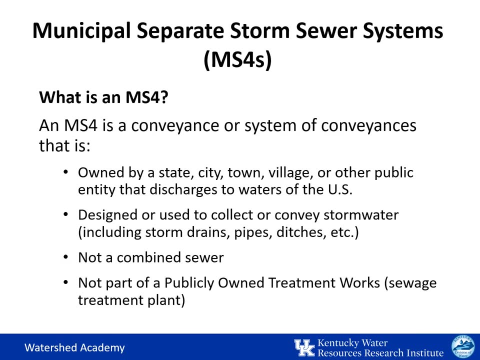 in 2006, in which there was a $500 million fine, and it addressed CSOs and SSOs. In 2008, Lexington was fined $300 million and it addresses SSOs, as well as stormwater system Moving on from the sanitary sewage system. 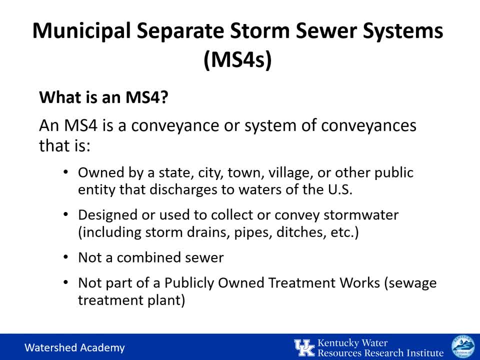 let's look more at the stormwater permits. We talked about separated systems and the MS4 is the name of the system that collects the stormwater separate from the sanitary sewer. It gets its names from M for municipal sewer and M for municipal sewer. 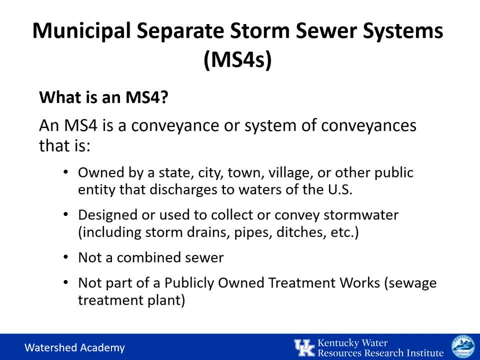 It gets its names from M for municipal sewer. It gets its names from M for municipal sewer. It gets its names from M for municipal sewer And four S's separate storm sewer systems. So this is owned by a state, a city or town. 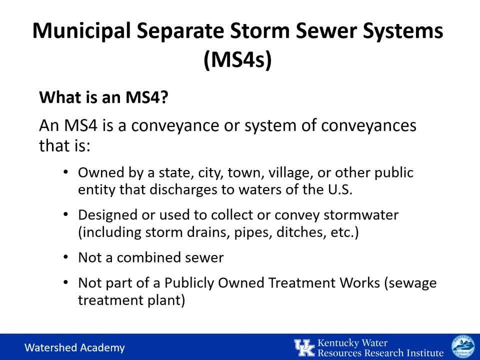 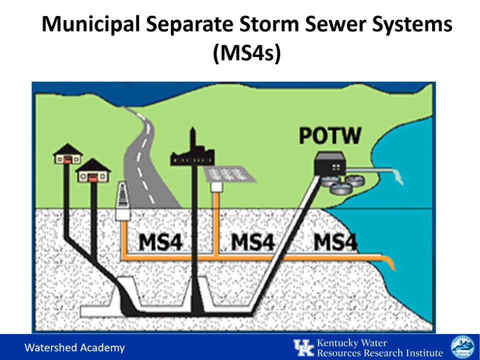 that discharges into the waters of the US. It's collecting the stormwater and delivering it, but it's not combined and it doesn't go through a treatment plant. So in this graphic we see a separated system in which the black lines represent the sanitary sewer system. 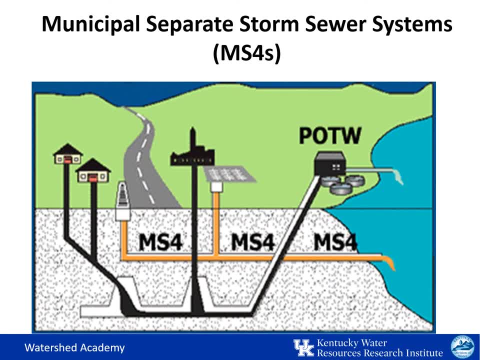 in which the black lines represent the sanitary sewer system which goes to the publicly owned treatment works or the wastewater treatment plant, And the orange lines show the storm sewer system or the MS4, in which the water is delivered untreated directly into the streams or other water bodies. 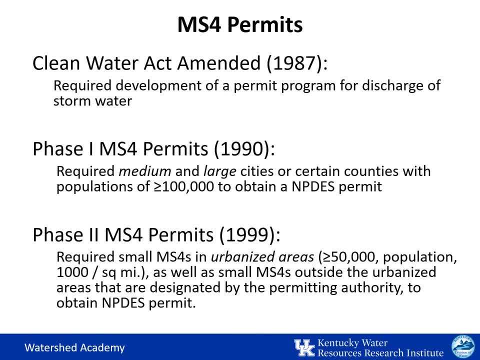 The history of stormwater permit is relatively short. The Clean Water Act was amended in 1987 to require the development of a stormwater permitting program. Phase I permits for communities with populations greater than 100,000s were required as of 1990.. 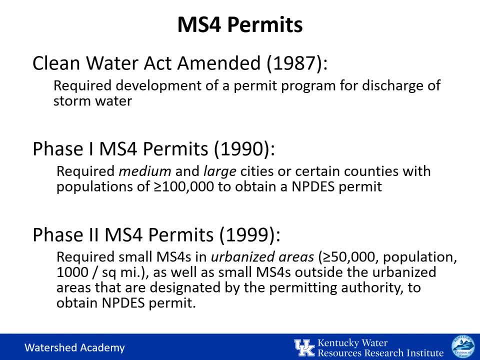 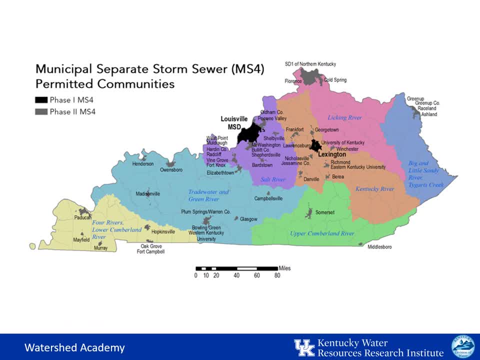 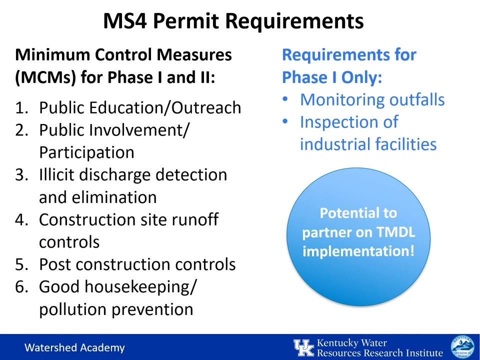 Smaller Phase II communities were required to have permits as of 1999.. This map shows the location of Kentucky's Phase I, that's, Lexington and Louisville, and Phase II, stormwater communities. Phase I and Phase II permits are similar in that they both have six minimum control measures. 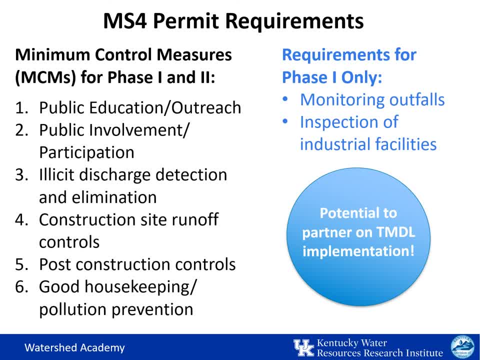 to be addressed. The Phase I permits are more specific and also require monitoring of outfalls and inspection of industrial facilities. These are individual permits. If you have an MS4 in your watershed, they can also serve as a great partner, particularly if you can align some of your activities. 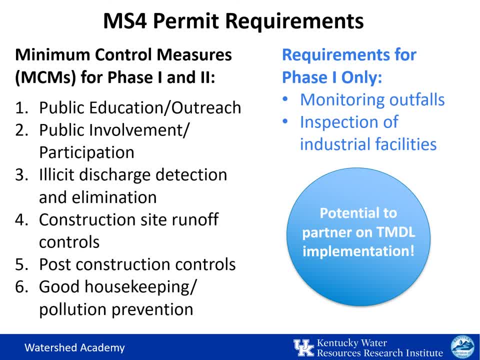 with requirements of their permits. All MS4s have public education and public involvement requirements. Therefore, they can be excellent partners when it comes to educating and engaging the public with regard to pollution problems in the watershed. MS4s also have post-construction control requirements. 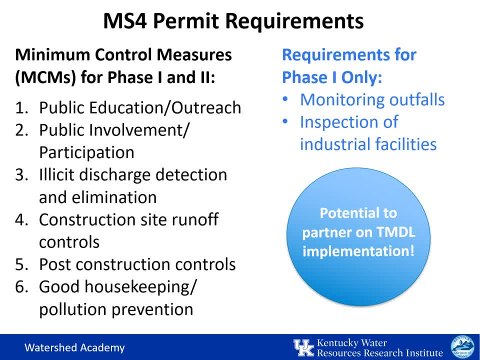 for stormwater retention and detention that are specific for each area. It is important to be familiar with these requirements. The pollution prevention requirements and prevention measure refers to specific controls for the municipal operation and facility, which will also be helpful to understand If a TMDL has been established in your watershed. 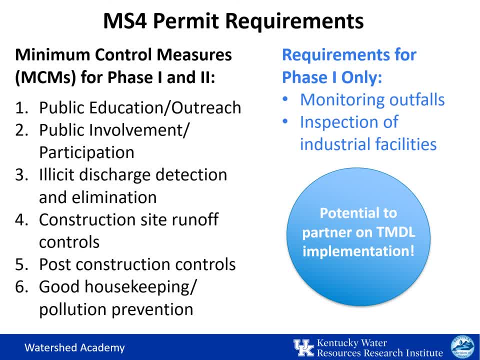 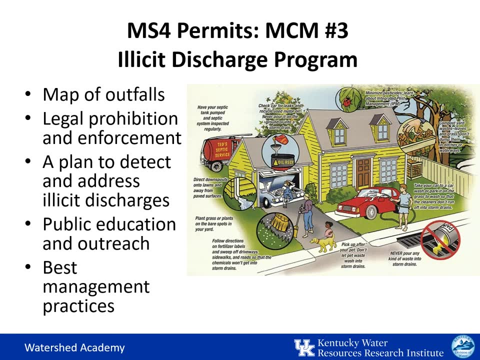 there may be opportunities to collaborate with the MS4 regarding its implementation. We will discuss some of these elements of the MS4 permit in more detail in subsequent slides. MS4s are required to have a program to identify and eliminate illicit discharges. Illicit discharges are generally anything other than stormwater. 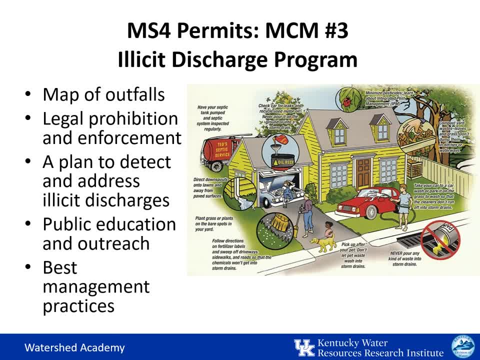 that is entering the stormwater collection system. Municipalities are required to map their outfalls so that they know how to trace illicit discharges through the system. They must have a plan to detect them, make them illegal through ordinances and have practices to address them. 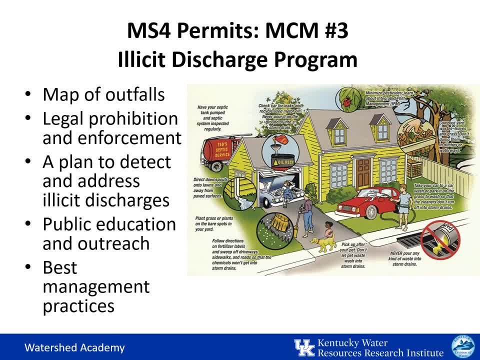 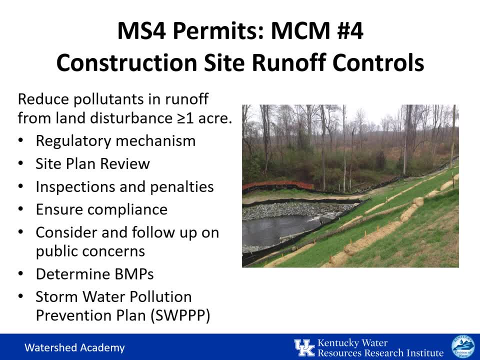 So MS4s can be partners in trying to track down some of these sources of pollution. if it occurs within their jurisdiction, MS4s must also inspect construction sites with more than one acre of land disturbance. This includes having a program to review site plans. 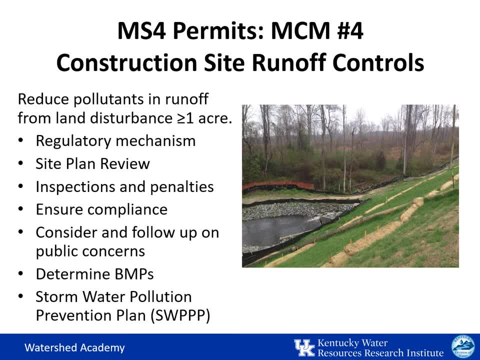 inspect facilities and ensure compliance. If you are working in an MS4 area and notice construction erosion problems, you may be able to work with the MS4 to resolve these issues. Each construction site is required to have a stormwater pollution prevention plan to address stormwater pollution. 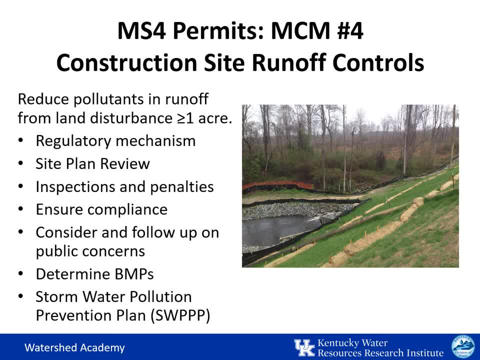 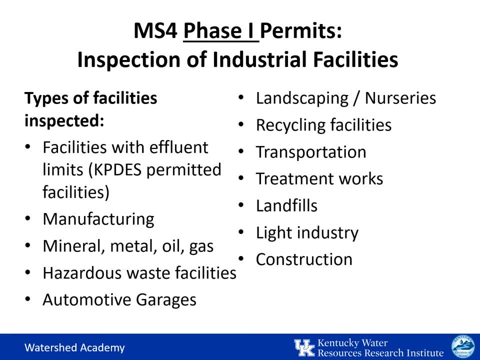 So if you notice sedimentation around a construction site, you should be able to work with the MS4 to ensure that the site comes into compliance. Phase 1 permits also require the inspection of industrial facilities to determine if they are contributing to water quality problems. 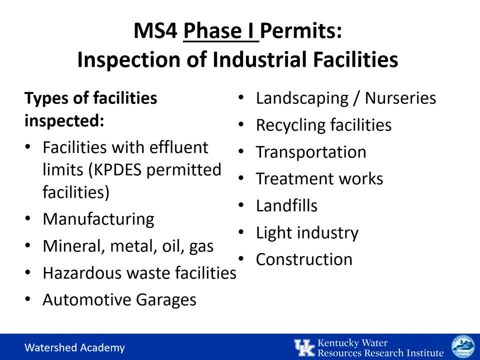 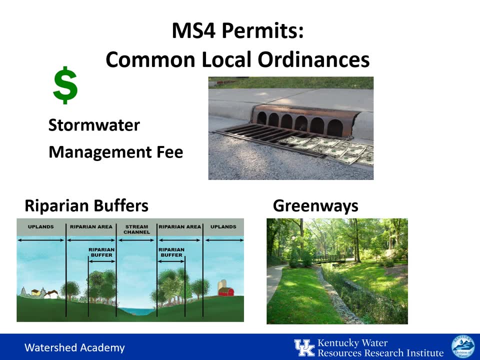 This slide lists some of the different types of facilities that might be inspected under this program. Again, this is for phase 1 permits and not for the stormwater pollution. If you are working in an area that has an MS4 permit, there may be some additional opportunities for working with the municipality. 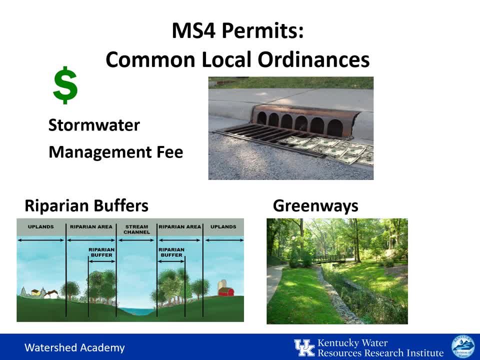 Many have a water quality management fee or a stormwater fee. This is usually based on the amount of impervious surface on an owner's property. This fee creates a fund that assists with the costs of implementing stormwater program and the installation of stormwater management. 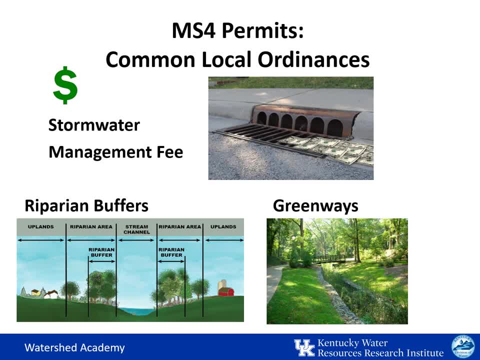 This is usually based on the amount of impervious surface on an owner's property. This is usually based on the amount of impervious surface on an owner's property. These fees may also be available for citizen-led BMP implementation projects or other uses, depending on the community. 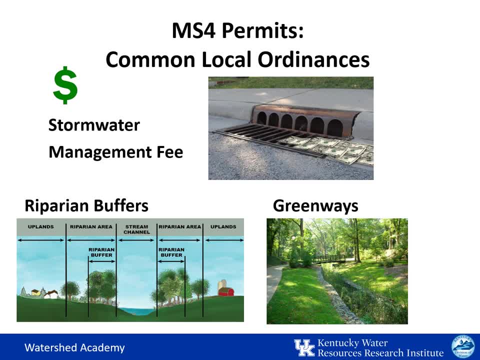 Check to see what the policy is in the area. Riparian buffers can also be an opportunity to collaborate. Communities may have ordinances or zoning requirements that protect Riparian Buffers by establishing a construction setback zone. We would like to thank each community for supporting this decision. 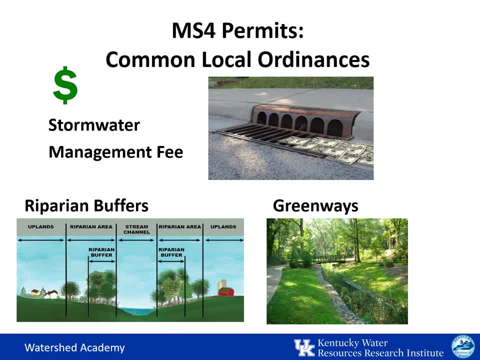 Some require the protection of a 25-foot setback from the stream bank. Greenways may also be an opportunity for collaboration. Greenways are corridors of open or natural spaces along stream that may be managed for conservation, recreation or wildlife protection. Management can vary from community to community. 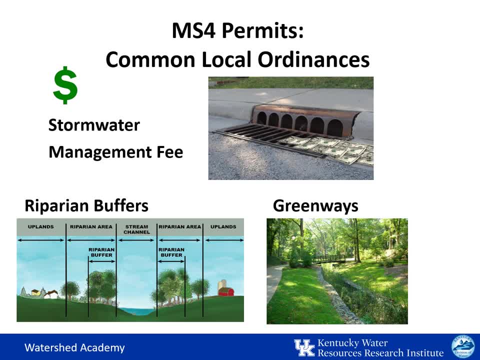 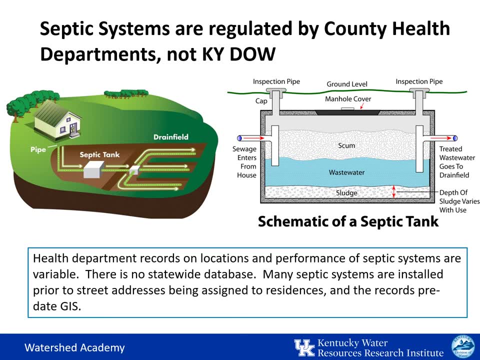 These greenway programs can have opportunities for water improvement in conjunction with recreational opportunities. We've talked about stormwater and we've talked about sanitary sewers, but in many areas of the state, sanitary sewer systems have not been constructed. Therefore, on-site wastewater treatment systems, primarily traditional septic systems, as well as some straight pipes, will be utilized to handle household sewage. 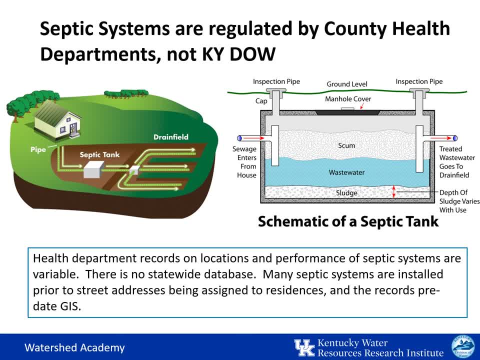 Septic systems work by allowing solid materials to settle out in the tank and effluent water to flow into the drain field, where it is then absorbed by the soil. The drain fields can become clogged with sludge and cause backups. These failing systems can contribute to in-stream bacteria concentrations, particularly if these systems are in close proximity to the stream. 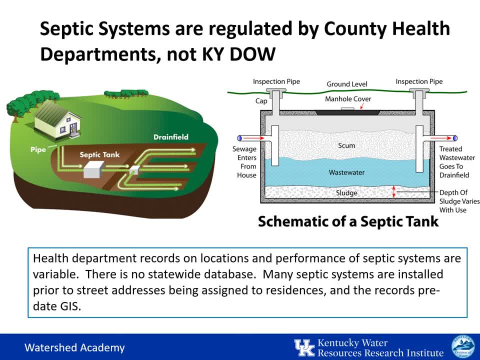 Soils throughout Kentucky are generally poor or inadequate for septic tank installation and sewage treatment. Karst features also enable sewage to flow more freely into the stream. This is due to the lack of adequate treatment of sewage and the lack of adequate treatment of groundwater. 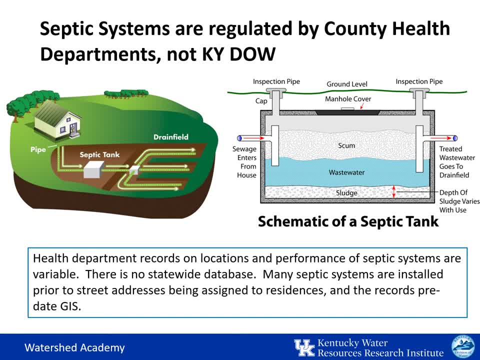 The Kentucky Division of Water does not regulate septic systems. These are managed by the county health departments. However, when wastewater is at the surface and running into a water body, it is a violation of 401 1031.. Watershed coordinators should know that there is not a statewide database for septic tank owners, nor is there even a county-specific one. 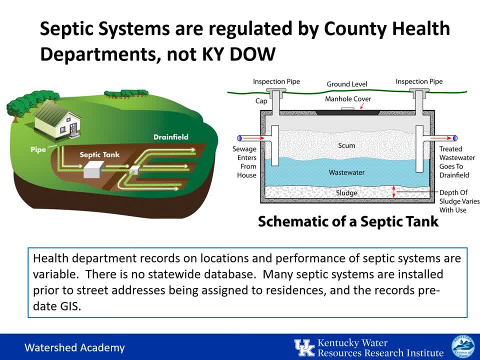 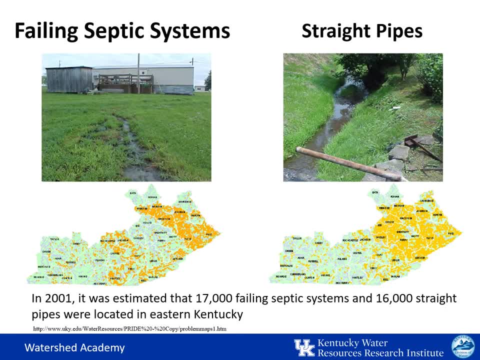 Records vary from county to county So you'll need to work with the county, The local health departments, to understand where problem areas might be Failing septic systems and even straight pipes are a huge problem in certain areas of the state where wastewater infrastructure has not been constructed. 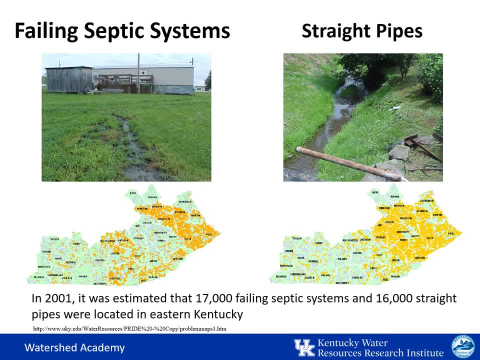 A 2001 study by Eastern Kentucky Pride and KWRI estimated that 17,000 failing septic system and 16,000 straight pipes were located in the area Through. although these figures have Likely decrease, this is still a huge issue for this area of the state. 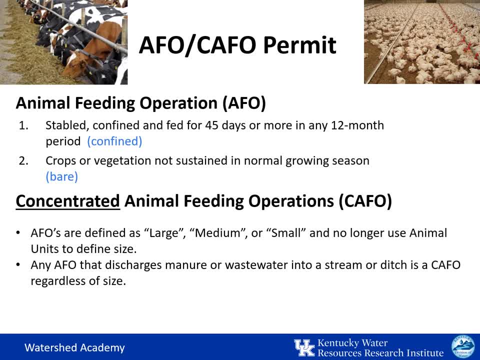 Not all animal feeding operations or AFOs are permitted, but operations with confined animals or confined animal feeding operations, CAFOs, are permitted. AFOs that are permitted have two things. They are confined, That is, that Animals are stabled or confined or fed 45 days or more in any 12 month period. 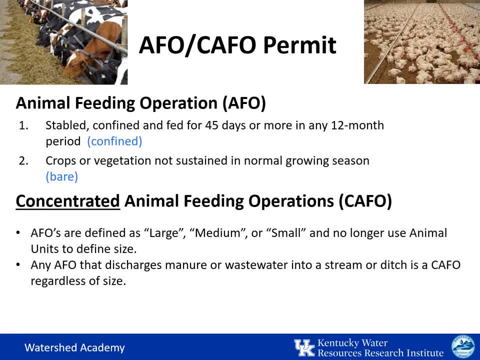 They also have bare ground. That is, that crops or vegetation are not sustained in a normal growing season. If it discharges manure or wastewater into a stream, then the facility automatically qualifies as a CAFO, no matter how big or how small. 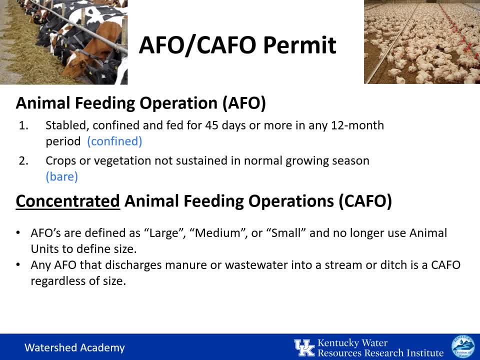 There are regulations defining CAFOs And AFOs. in 40 CFR 122.23. large animal feeding operations means that the AFO stables or confines as many or more of set numbers of animals, for instance 40 dairy cows or 1000 other cattle, 2500 swine, 500 horses. 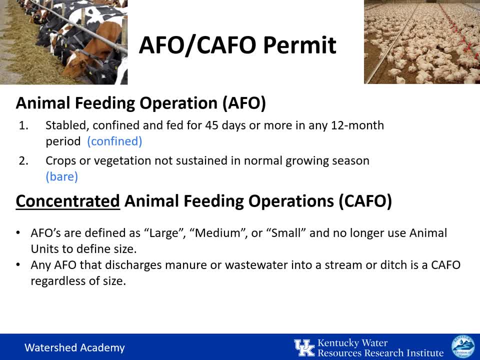 You can see the other descriptions that are In the law. a medium facility has 200 to 700 mature dairy cows, 300 to 999 heifers, and you can go down the list. So, based on different amounts of size, they may be categorized at these different large, medium or small levels. 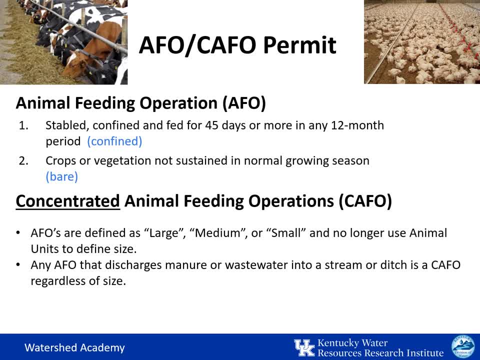 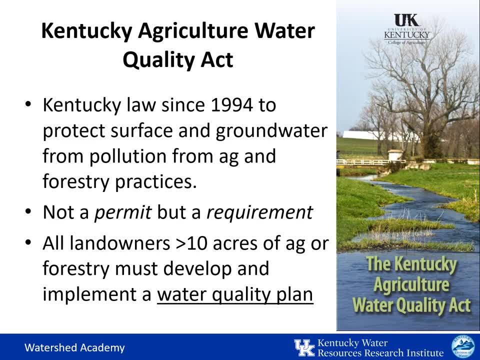 But the point is they have confined animals and bare ground and Any discharges of manure, of waste, into the streams. The Kentucky Agricultural Water Quality Act is not a permitted system, but it requires all landowners with more than 10 acres of agriculture or forest land to develop a water quality plan. 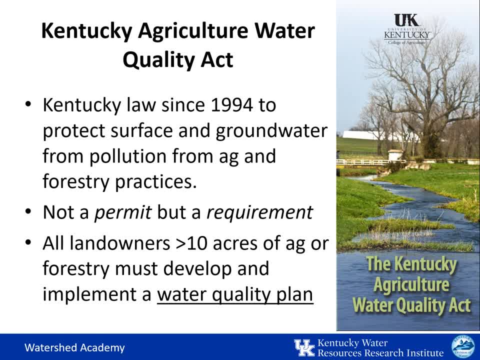 The water quality plan specifies best management practices related to forestry, pesticides and fertilizers, farmsteads, crops, livestock and protection of streams and other waters. It is a way to help farmers ensure that they are protecting waterways as they can host their farming operations. 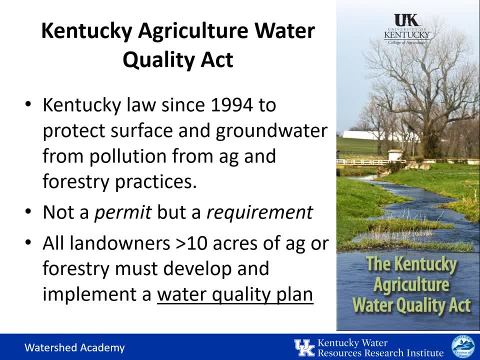 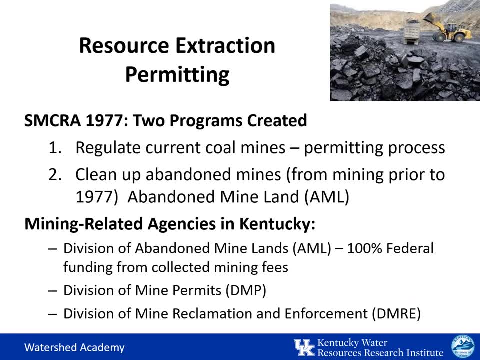 Farmers must provide their plan in order to qualify for cost sharing assistance through federal farm programs. The surface mining control and Reclamation Act, also known as SMCRA, in 1977 created two programs: one regulated, current minds for being a permitted process, and the second 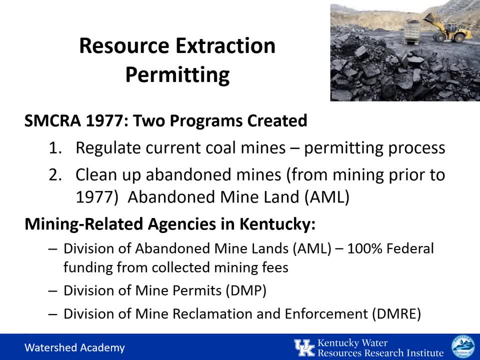 Cleaned Up Abandoned Mines. The Division of Abandoned Mine Lands, or AML, works throughout Kentucky's coalfields to protect the public from health and safety problems caused by mining that occurred prior to 1982. AML administers a water supply replacement program through which they extend water lines. 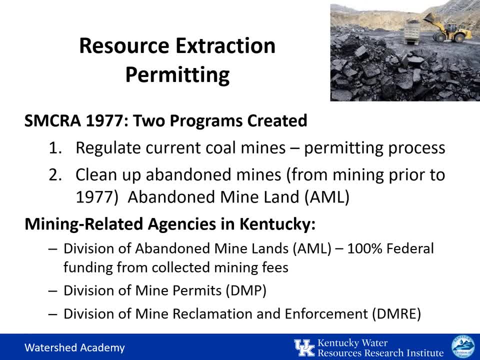 into areas where drinking water has been contaminated by past mining activity. The Division of Mine Permits ensures that permitted activity meets the human health and environmental standards of SMCRA. The Division of Mine Reclamation and Enforcement is responsible for inspecting all surface and underground coal mining permits in the state to ensure compliance with SMCRA. 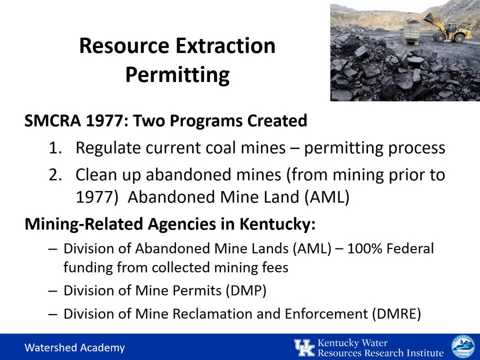 Also responsible for regulating and enforcing laws for non-coal mining sites, including extraction of limestone, sand, gravel shale and river sand and gravel. Sections 401 and 404 of the Mining Act are the following: Section 401 and 404 of the Mining Act are the following: 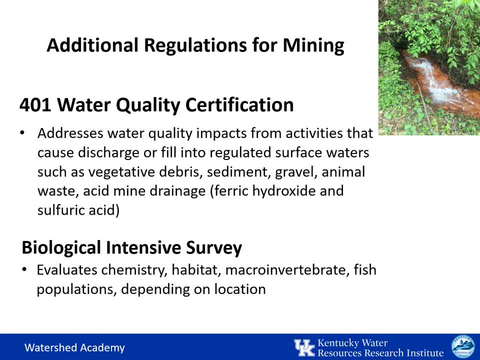 Section 401 and 404 of the Mining Act are the following of the Clean Water Act regulate projects that involve the discharge of dredged or fill material into waters of the United States. This applies to any type of dredge or fill material, but mining activities creates dredge and fill. 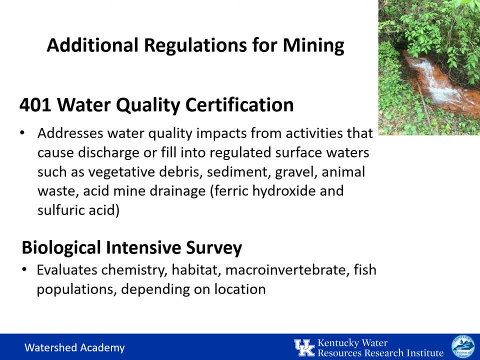 materials and therefore it is covered by the 404 permitting and 401 certification requirement. This certification includes management requirements for handling vegetated debris, sediment and acid mine drainage created through the mining process. The next slide will provide additional information on 401 and 404. 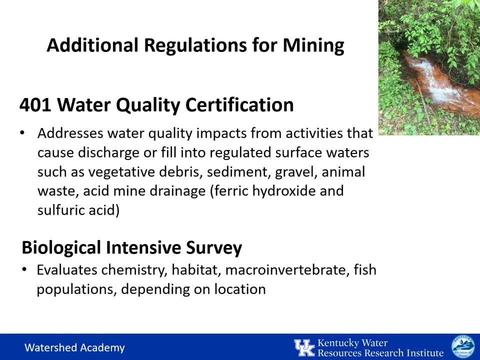 requirements. A biological intensive survey is also needed for coal mining permitting. The Kentucky Division of Water has specific guidelines for sampling and site of identification that are published on its website in order to guide what mining operations are required to sample. The guidelines require chemical samples as well as different types of 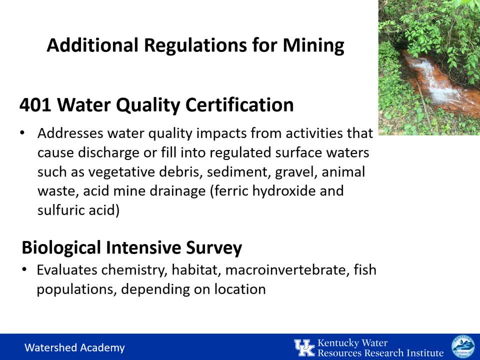 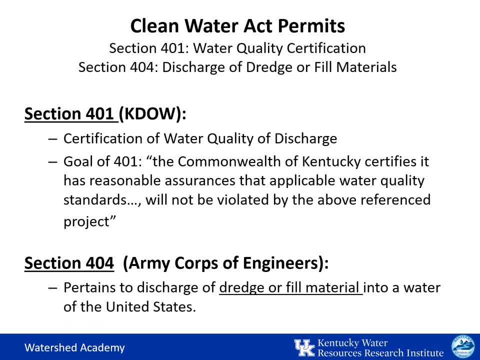 biological samples, depending on the size of the waterways. For construction permits that will potentially impact a water of the United States, two different permits are needed. The Army Corps of Engineers administers the 404 permit process, as we previously discussed. The applicant must perform a 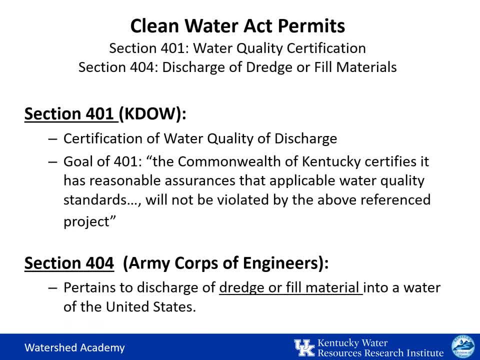 jurisdictional determination of all water resources in the construction area. This means determining whether there are any streams or wetlands in the area and, if so, determining their size or length and how much would be impacted. there are then required to assess whether these water resources are a water of the. 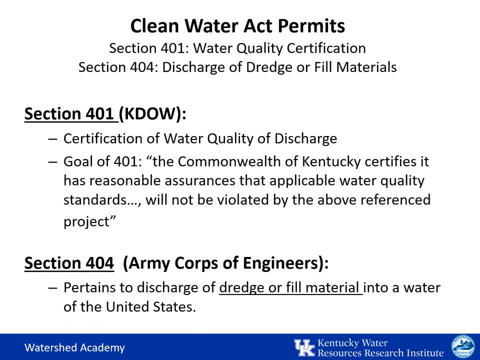 United States in conjunction with the permitting agency. the Kentucky divisional waters 401 certification validates the US Corps of Engineers 401 permit. 404 permit. this dual agency approach ensures that the federal and state regulatory agencies approve of the projects and have outlined their expectation for measures that will protect water quality. 404 permits or. 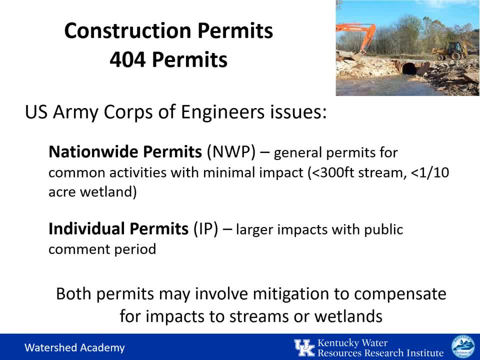 construction permits are issued generally in two different types: nationwide permits and individual permits. nationwide permits are general permits for common activities with minimal impact, that is, less than 300 feet of stream are impacted or less than a tenth of an acre of a wetland. some common nationwide permits include: 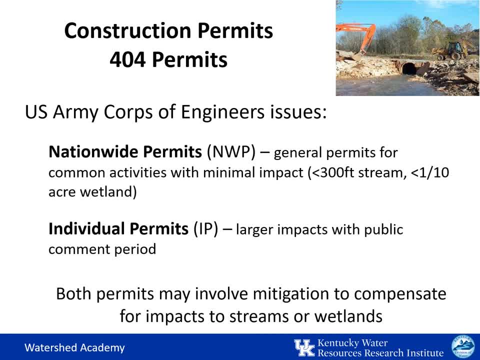 number three maintenance activities, 12 utility lane crossings of streams, 13, which is bank stabilization, 14 road crossing of streams, 21 surface mining activities, 27 stream and wetland restoration and and water conservation and water conservation and water conservation, and 39 development. individual permits are larger impacts with the comic with a. 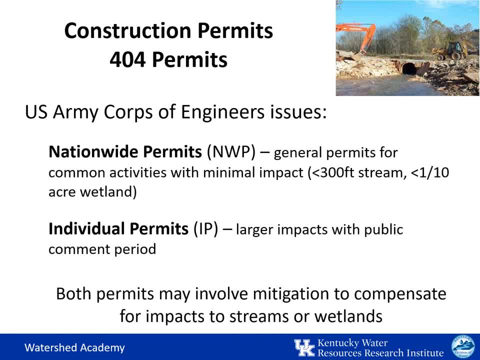 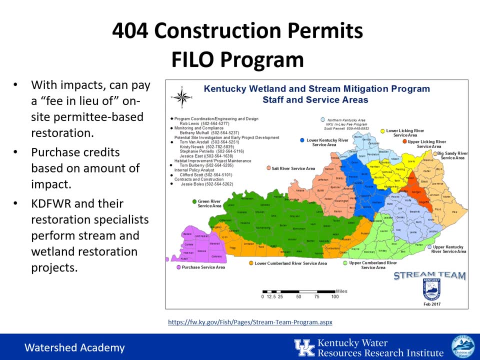 public comment period. both permits may involve mitigation to compensate for impacts to streams or wetlands that result as part of the construction process. when significant impacts occur, the permitting can mitigate them by restoring a stream or wetland in another area, or they can pay a fee in lieu of 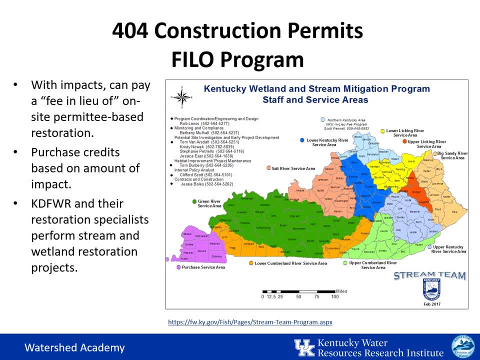 conducting services for a water rig or paths that are faulty or part of government the restoration themselves. these fees are then used to professionally restore a stream segment or wetland area within the same river basin as the construction project. this fee in lieu of program or philo is managed by multiple agencies but is directly overseen by the kentucky department of. 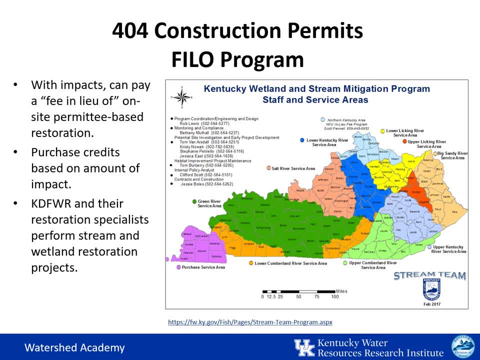 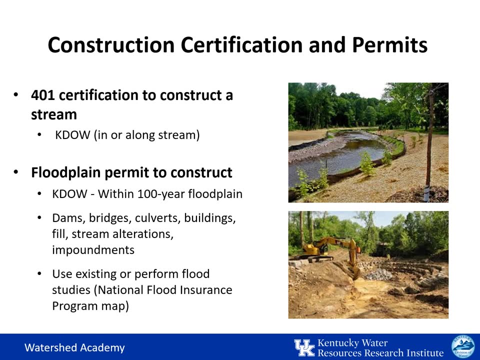 fish and wildlife resources. the philo program is provided for in krs 150-255. permits are also required from the division of water for stream construction, and that includes stream restoration work as well as construction activity within the 100-year floodplain. the 100-year floodplain is the land that is predicted to flood during a one-hemp. 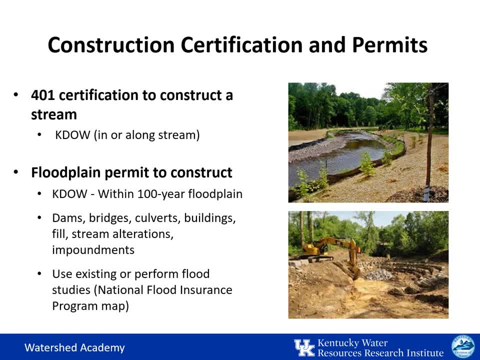 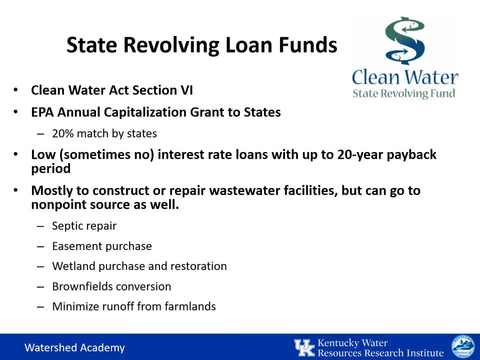 100-year storm. it has a one percent chance of flooding during even any given year. title six of the clean water act provides for state revolving loan funds. through this program, the epa provides annual annual capitalization grants to state requiring 20 match by the states. 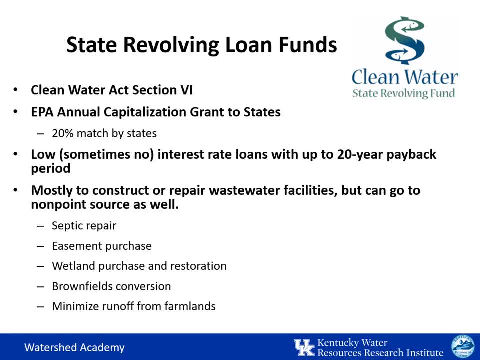 these low, sometimes no interest. late loans have a 20-year payback period and can be allocated to the kentucky department of fish and wildlife resources. the kentucky department of fish and water land is also required for the plan for the project to be reviewed, and under a 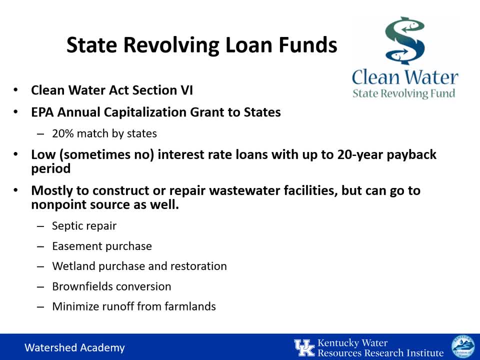 wire fee of 60ят a year by each state or region that has the right of way to include 250 bet. so, as a part of the urban development project, the kentucky department of fish and water and the food industry, the kentucky department of fish and water have all the same requirements. that the kentucky department of fish and water have to meet for the land and water. this diagram shows how funds flow in the state revolving law eart. in addition to green water project funding programs, there are several types of projects, such as green waste- waste water infrastructure. 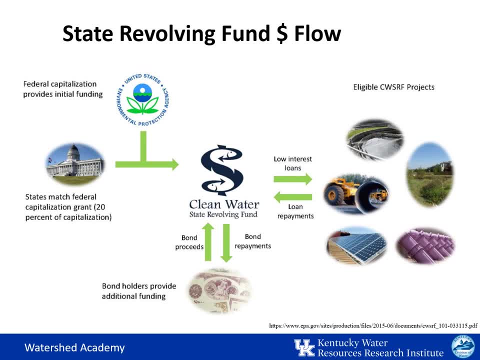 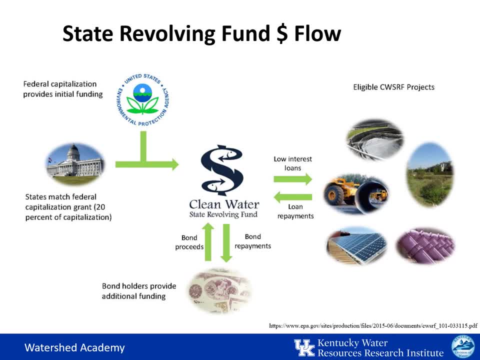 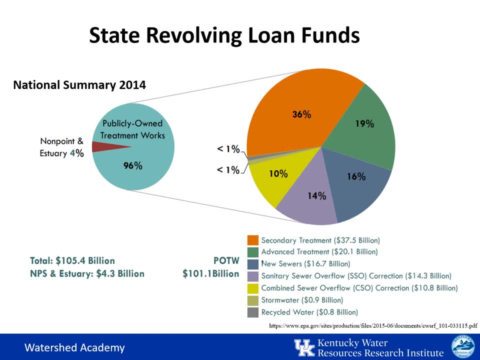 interest loans on the amounts to complete their projects. these pie charts summarize how SRF funds were used nationally in the year 2014. by far the majority of funding was used for wastewater treatment plants and related infrastructures, though down point sources and estuaries were funded at 4%. 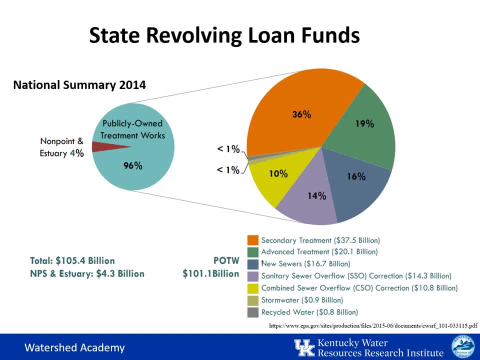 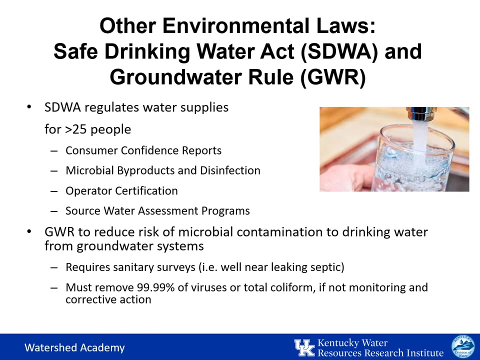 of the total infrastructure. you can see a lot of the money goes towards secondary treatment as well as advanced treatment: 16% towards new sewers and another 14% towards sanitary sewer overflows and 10% towards combined sewer overflow Corrections. often when the public thinks about water quality, 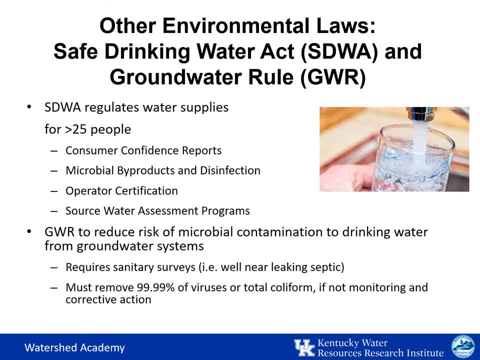 protection, they immediately think not of streams, but of drinking water. it is important to know that the Safe Drinking Water Act, or SDW a, and the groundwater rule, or GW, are our legislative mandates that are in place to ensure that water quality is maintained and that water is. 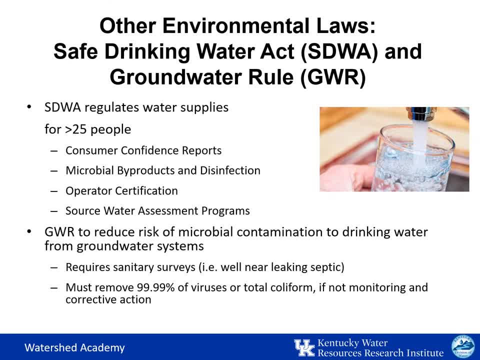 protected by the public and the state's public and local government. these laws help ensure that the public understands the quality of their drinking water and any contamination concerns a water body could be failing standards required for recreational use, but still provide quality drinking water after treatment and disinfection. the SDW a requires consumer confidence reports. 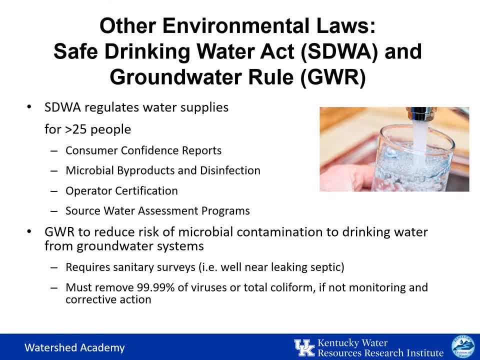 that you receive in the mail and they have rules about disinfection by products, potential contamination, threats to the water supply and operator certification that are reported in these reports. the groundwater rule includes additional requirements for the protection of drinking water systems that use groundwater sources. it also requires surveys for potential contamination. 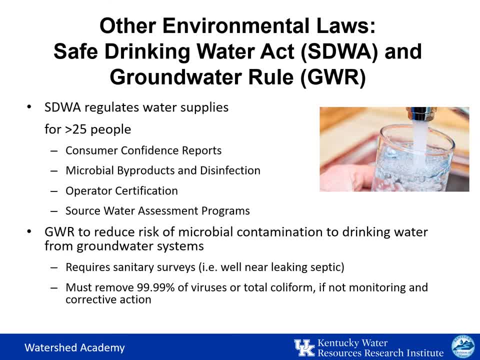 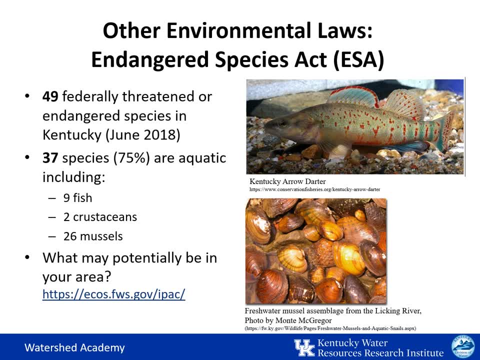 sources and calls for corrective action if viruses or bacteria are present. the Endangered Species Act has produced an annual dashboard. the SDW a is for requires that federal agencies ensure that their activities are not likely to jeopardize the existence of threatened or endangered species, If these 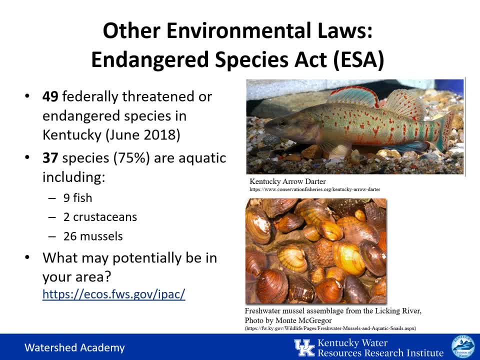 species are present in your watershed. they may restrict some of your planned projects, but they may also provide opportunities to create protected habitat for the species. There are 49 federally threatened or endangered species in Kentucky, and 37 of these species- that is, 75%- are aquatic species. 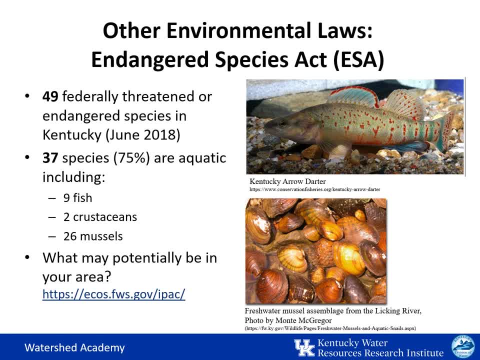 including nine fish, two crustaceans and 26 mussels. If you want to have more information about what is located in your area, please see the link that's located in the slide. The last of the other environmental laws that we want to. 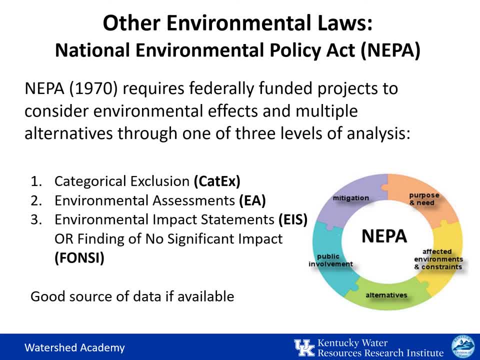 look at today is the National Environmental Policy Act, or NEPA. NEPA was passed in 1970 and requires federally funded projects to consider environmental effects and multiple alternatives through one of three progressive levels of analysis. A categorical exclusion is for projects that don't, individually or cumulatively 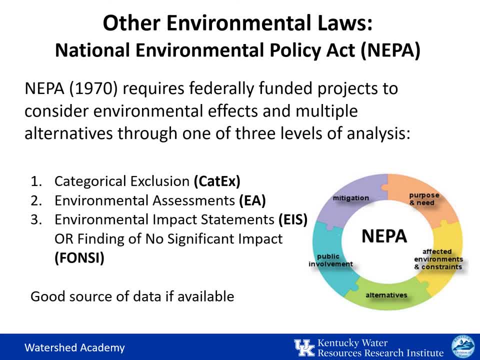 have a significant environmental effect. Environmental assessments, or EAs, assess whether or not the project has potential to cause a significant environmental impacts. It addresses the need, the alternative, the impacts and consultation. An environmental impact statement or a finding of no significant impact require more rigorous and detailed. 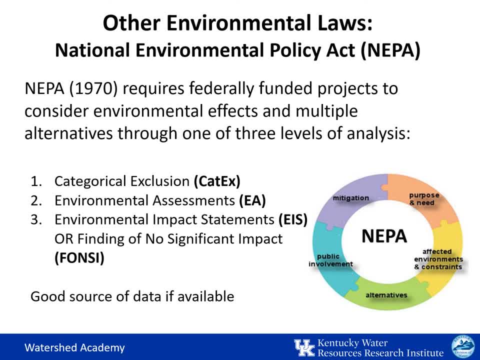 documentation with public comment explaining different decisions that were made along the way. The more rigorous the document, the more detail that may be available. As a watershed coordinator, these documents may have done a lot of the work for you. They typically consider the following impacts and provide related discussion that is affected environment. 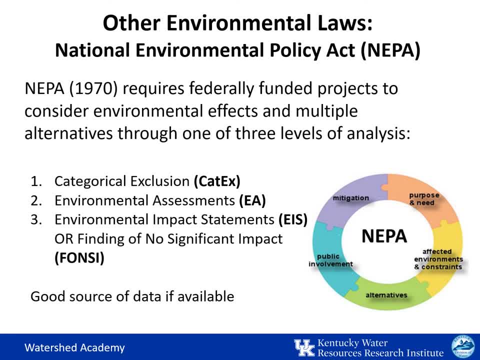 threatened and endangered species, air quality, water impacts, historic and cultural preservation, socio-economic impacts, soils and geology, noise and esthetics, energy, hazardous waste, direct, indirect and cumulative impacts and cost analysis. So, if there's a federally funded project in the watershed area, such